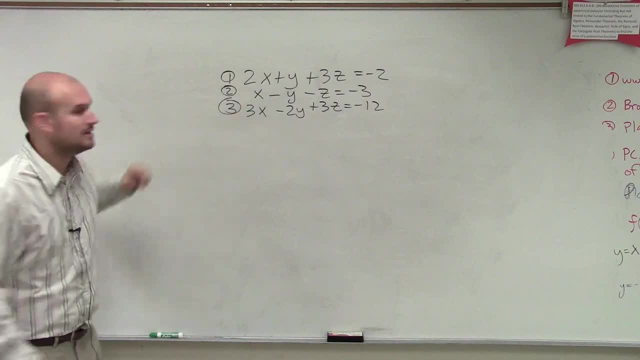 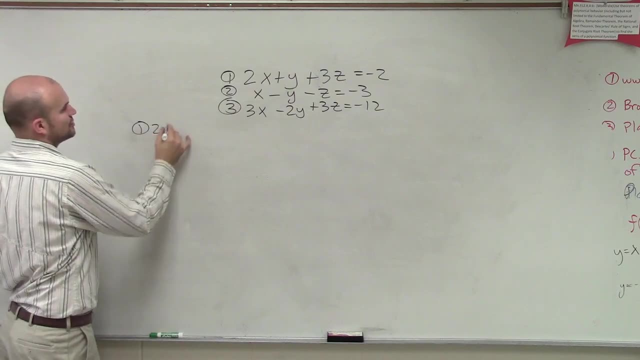 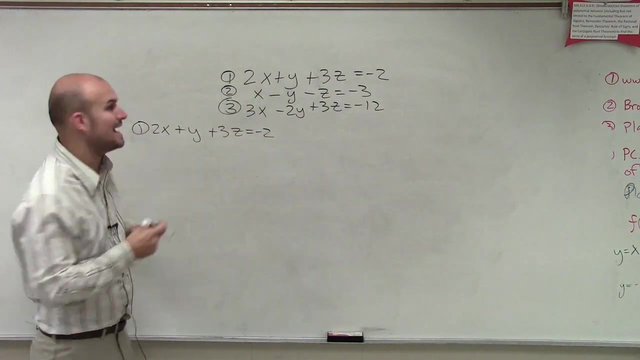 I can multiply this by a multiplier of negative two, right? So let's take an equation, number one and number two. So for equation one, I have 2x plus y plus 3z equals negative two. However, I am going to to eliminate the x. 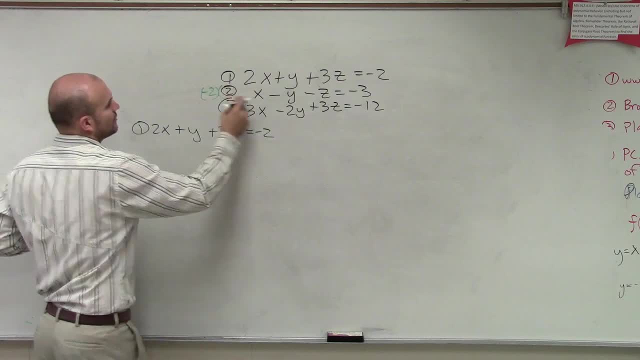 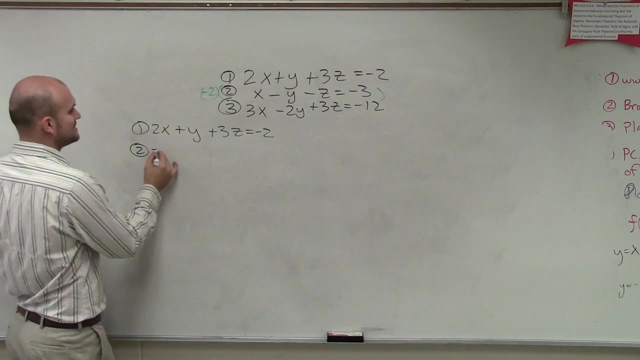 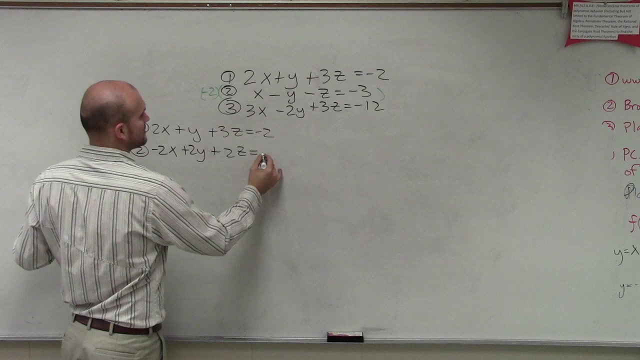 between one and two. I'm going to multiply equation two by negative two, Alright, So when I do that, equation two now becomes negative. 2x plus 2y plus 2z equals positive six. Has everybody followed me with that? 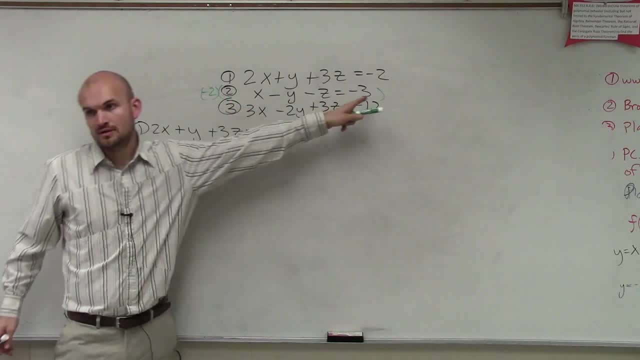 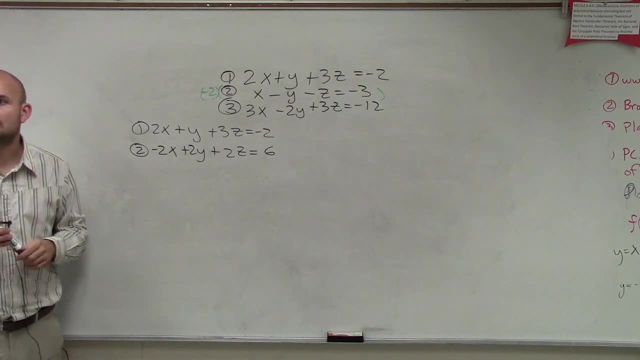 Oh yeah, I multiply negative two times. my second equation: Yeah, Yes, Can you just use y as a sum? Mm-hmm, You could have just added them up together. yes, But we asked to use the x variable, so I'm doing a sum for x. But yeah, if you wanted to use y, then you could. 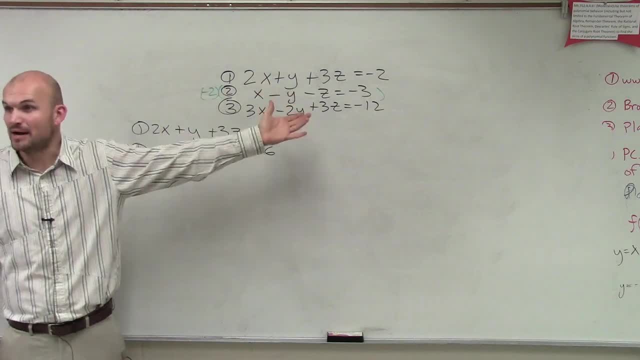 have just added the two equations up right, You didn't even need to multiply by a multiplier. Yeah, That would have been- probably would have been simpler for the first two, but it might not have been simpler for the next two. So I'm going to do a sum for x. I'm going 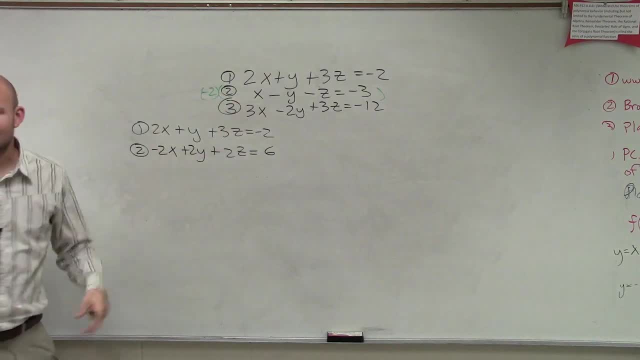 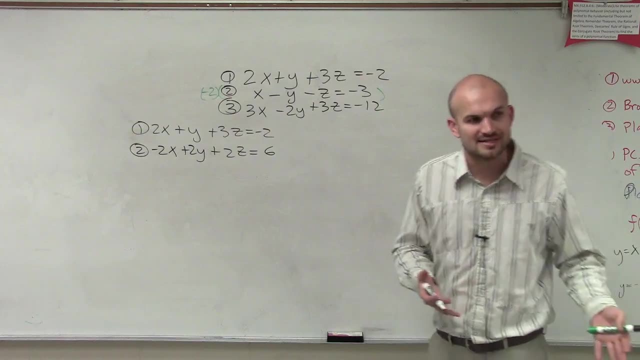 to do a sum for the next two. I don't know. Well, I do know, but I'm just trying to go through it. as far as a student would go, It doesn't matter what you pick. One might be easier than the other, but as long as you follow the same process, it's okay. You don't? 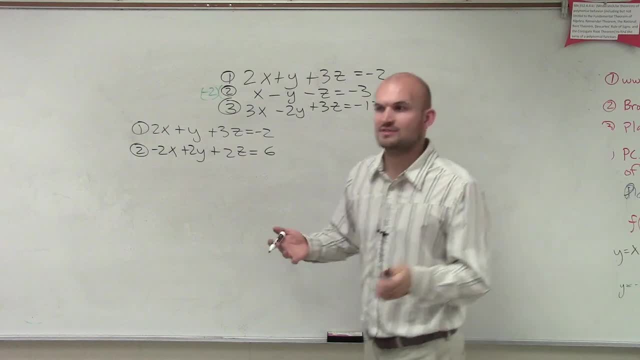 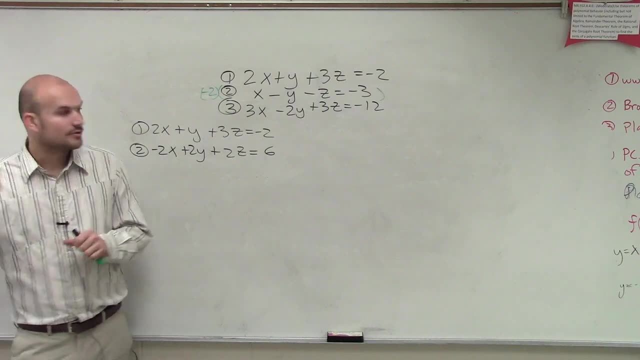 have to like get stressed out if, like, oh, is this the right one or not? They're all correct. Some might be a little bit easier, though than others. Yes, Why would you multiply the equation by two? The reason why I multiply by two is because now I have a positive 2x and a negative 2x. 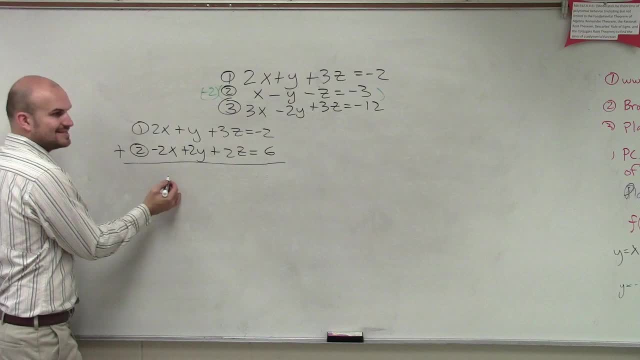 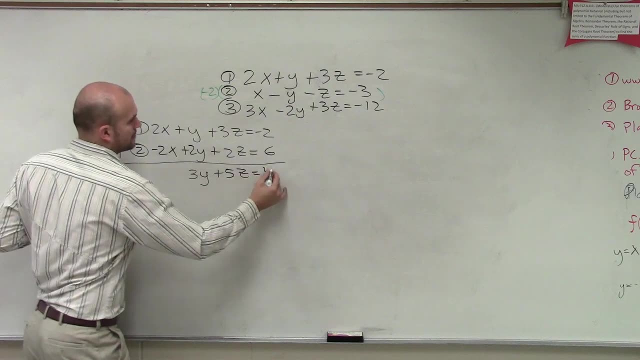 So when I take these two equations and add them, I now get a 0x, which means my x's have now been eliminated. Does that make sense? So what Dylan was saying is: why don't you just add them up? Well, I could have, but the student. 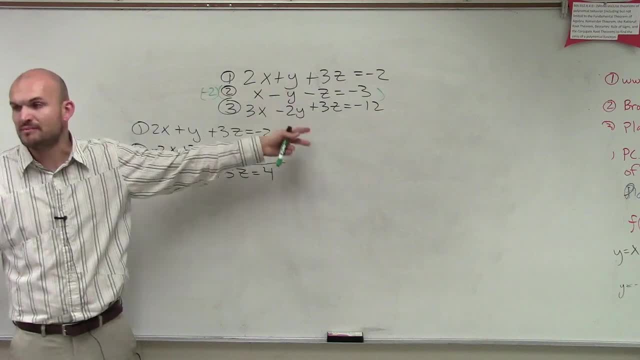 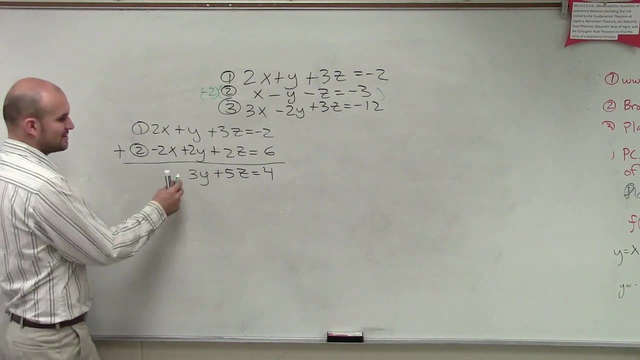 told me to eliminate the x's, But if you just would have added them up, then you would have eliminated the y's, which is okay too. It doesn't matter, It's okay Whichever way you see it, and you want to roll with it, that's fine. So we take our resulting equation and 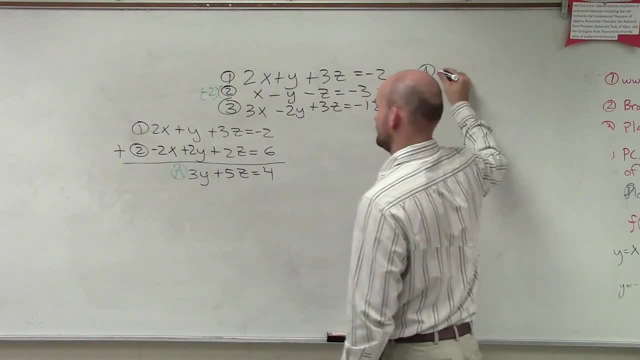 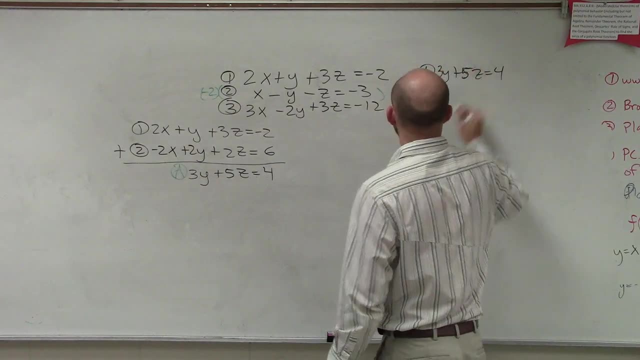 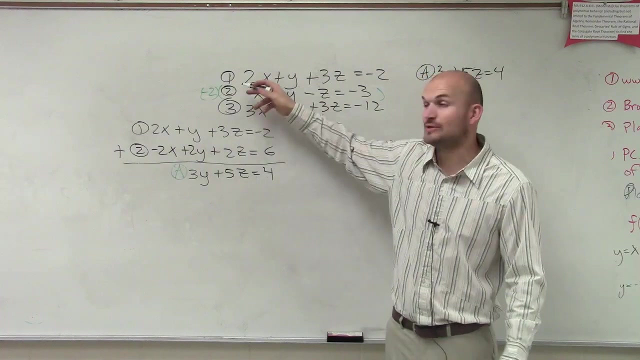 I say that I'm going to label that as a. So I write a A over here. A is 3y plus 5z equals 4.. Now the important thing to do, ladies and gentlemen, is, once you eliminated x between the first two, you now have to eliminate x between the. 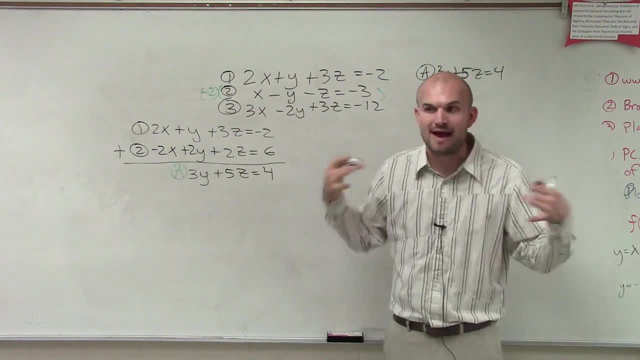 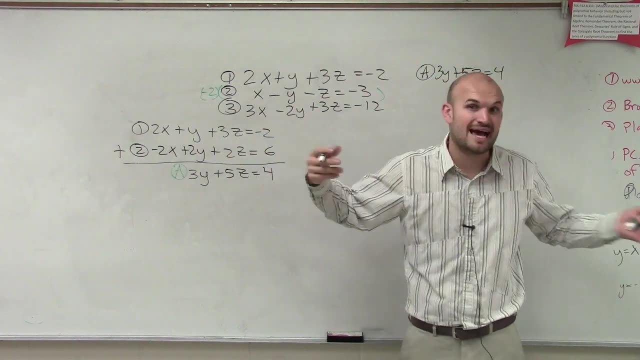 second two. So you can't eliminate x and then eliminate y. You have to remain consistent. So even though it might be easier to eliminate y in the first two, it might be easier to eliminate x in the other two. You just can't say, oh, whatever, one's easiest for one is: 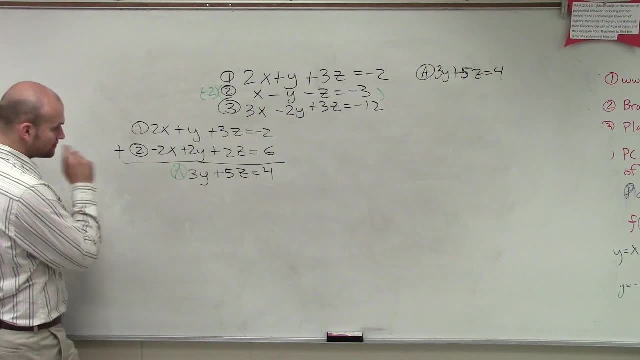 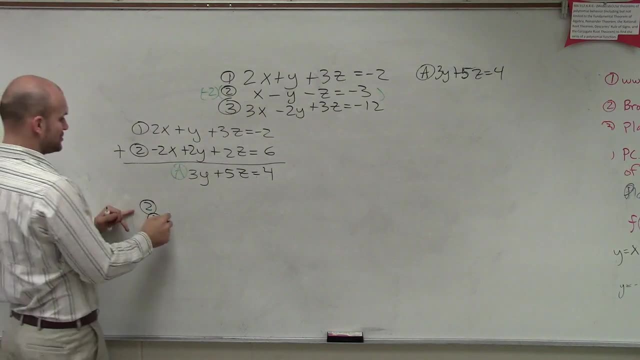 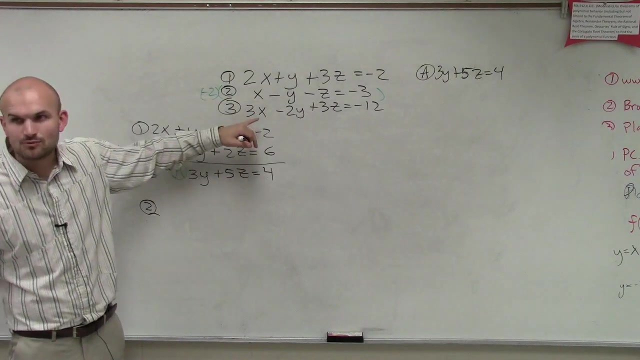 always going to be the easiest equation. So now I'm going to take equation 2 and equation 3.. So equation 2, well, let's write out equation 3.. All right, So, between equation 2 and equation 3, to eliminate x, what do I need to do to? 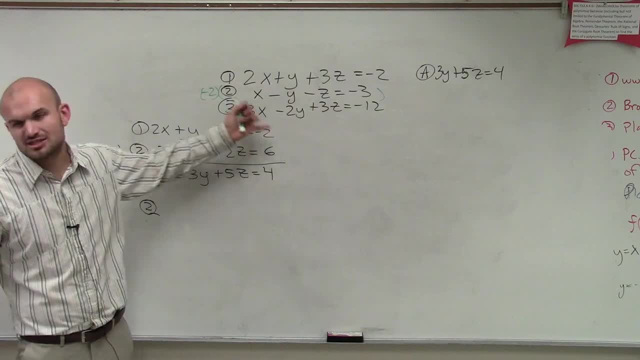 equation 2?. Multiply it by 3.. Multiply it by- let's call it by my negative 3. this time right, Because if I multiply it now by negative 3, I'm now going to get a negative 3x plus. 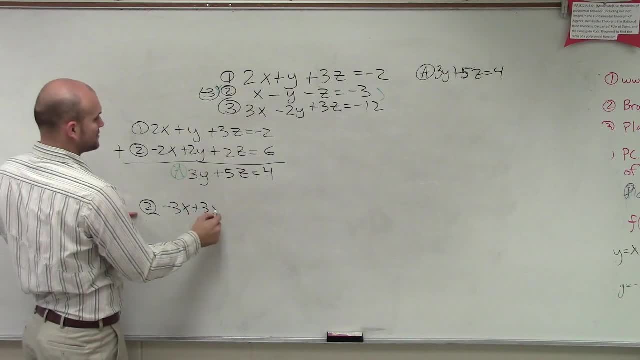 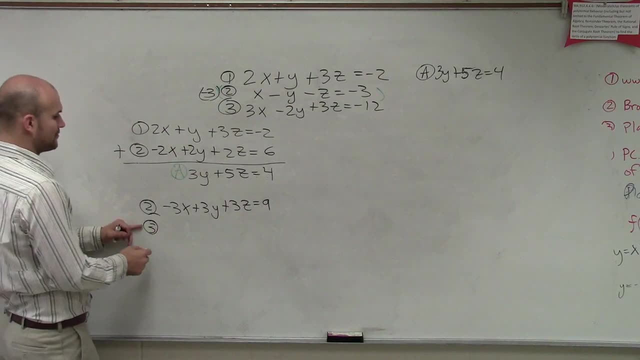 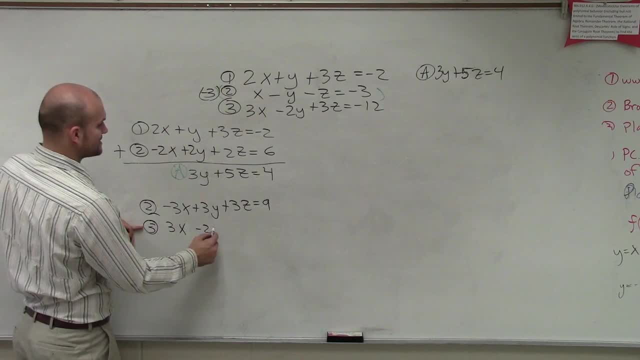 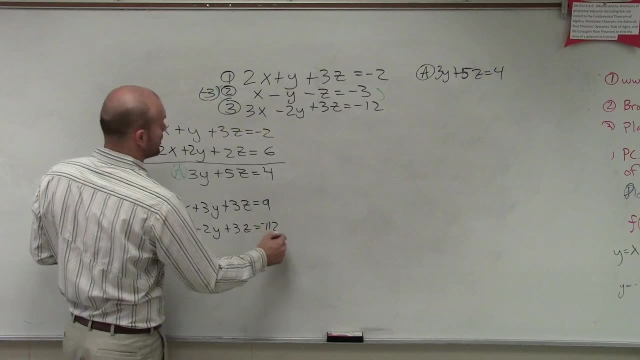 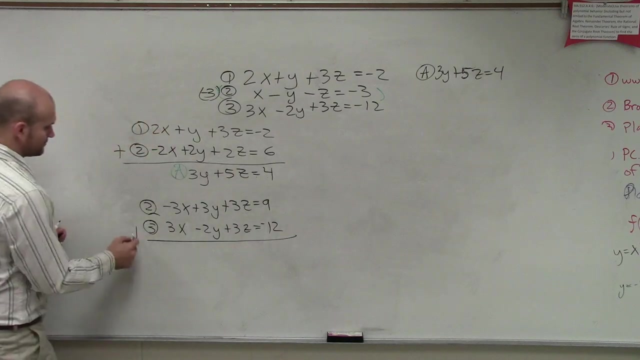 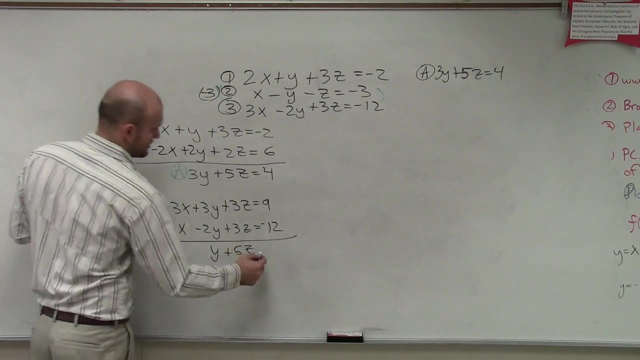 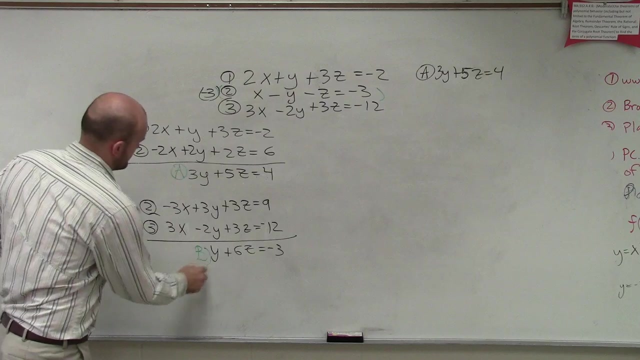 which will be 3x minus 2y plus 3z minus, equals negative 12.. That's 112.. So now I add these up and again I eliminated my axis. I get y plus 6z equals negative 3. So I call that equation b. 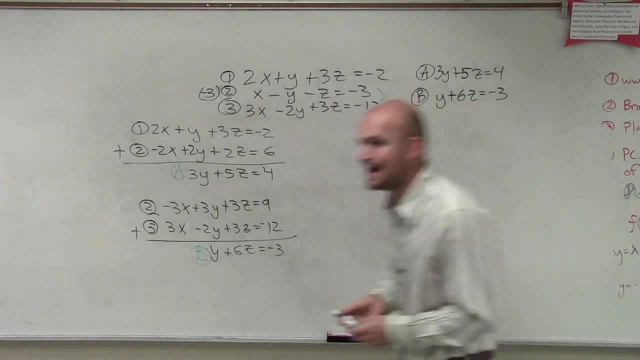 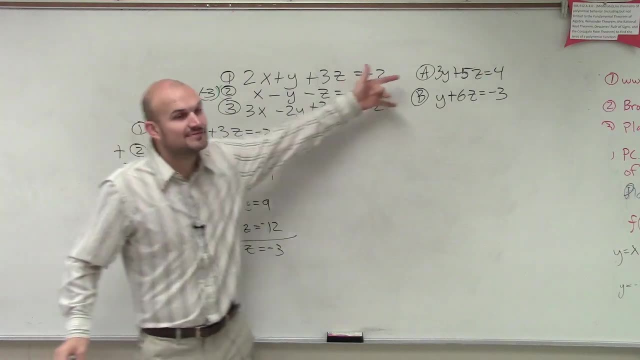 Okay, so now, ladies and gentlemen, we have two equations with two variables. Let's see, Let's see, Let's see, Wendy, do you see that When you have two equations with two variables, now what is so important? Now, what we can do is we can use elimination. 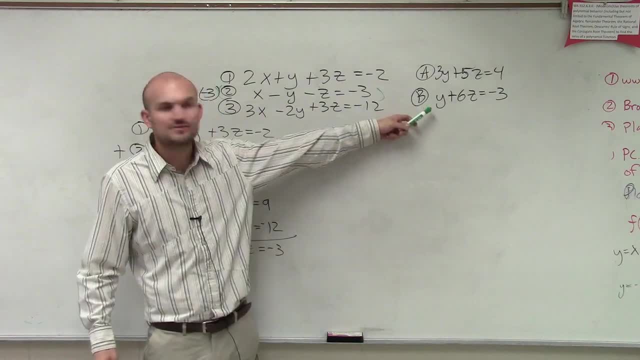 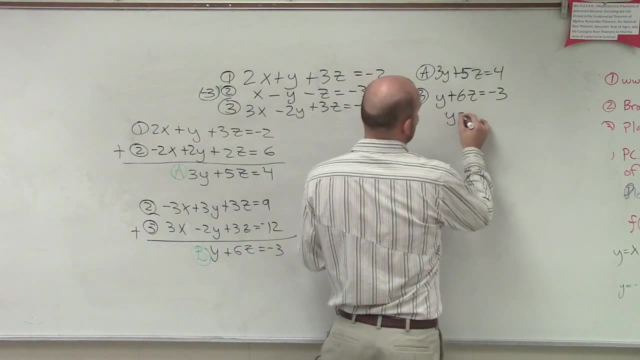 substitution. whatever you want to do, I would probably say, oh, let's use substitution, Let's substitute y, Let's solve for y and substitute it in. So I could say: y equals negative 3 minus 6z. Plug that in, You have 3 times. 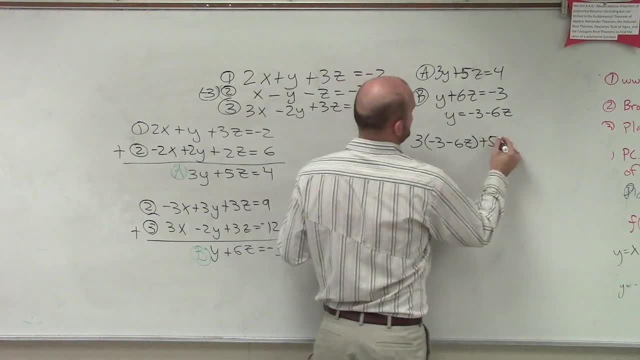 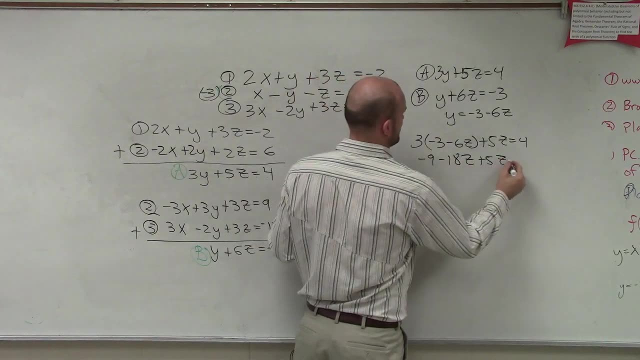 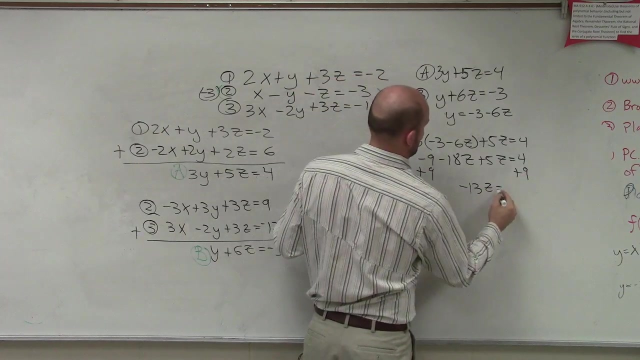 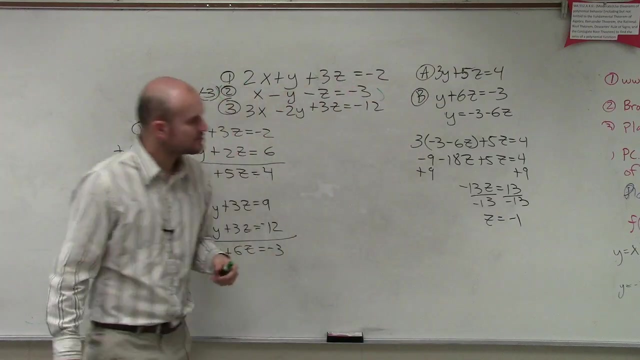 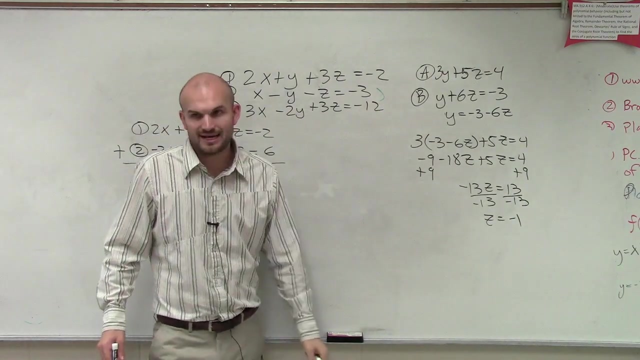 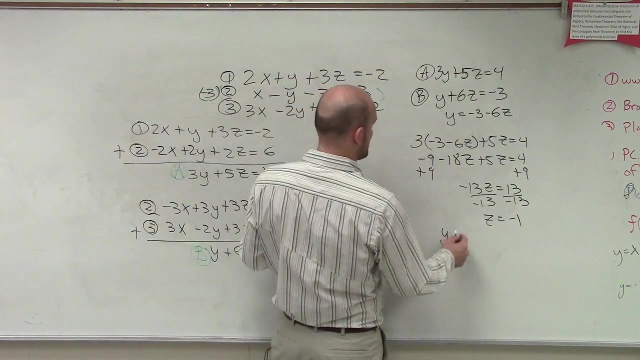 negative. 3 minus 6z plus 5z equals 4.. So when I plug in, when I solve b for y equals for y, I plug it into the other equation and I eliminate. I get z equals negative 1.. Now, since I know it, z is, now I can plug in negative 1 in for z. 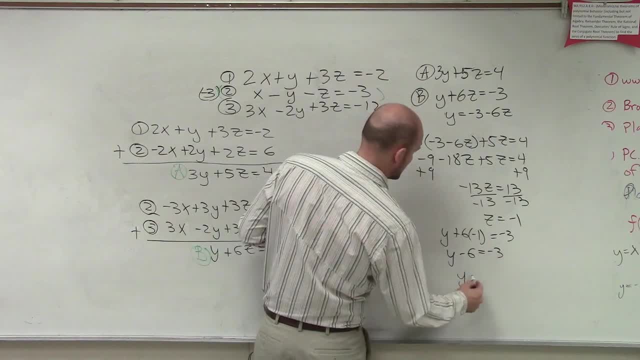 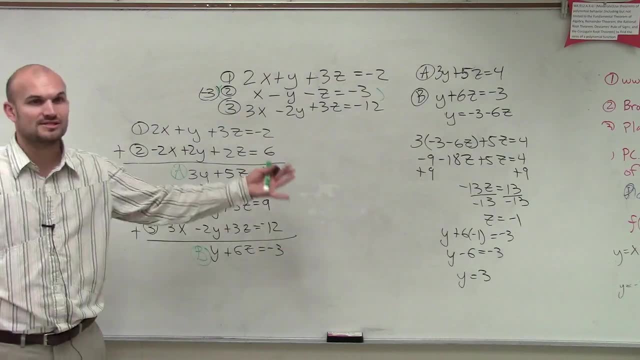 And I get: y minus 6 equals negative 3.. y equals 3 when I solve there. So now, ladies and gentlemen, once I know what y is and once I've already solved for z, So do you guys see how putting it in two systems, two equations, helps you find these two variables? 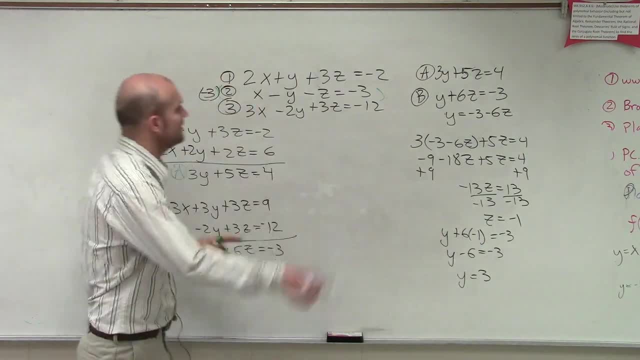 So now, once you know the value of two variables, all you need to do to find the third is plug them back into one of these equations, And it doesn't matter which equation you guys want to plug it in, for I'm going to pick this one because it has 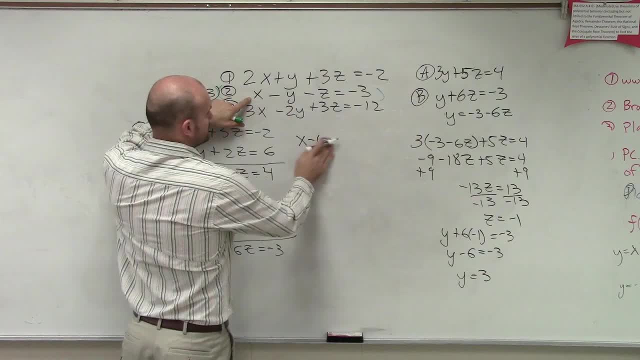 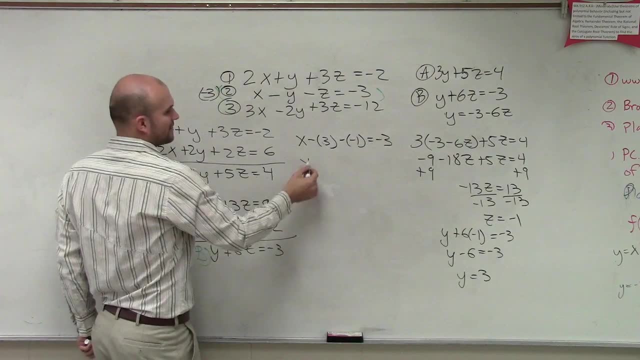 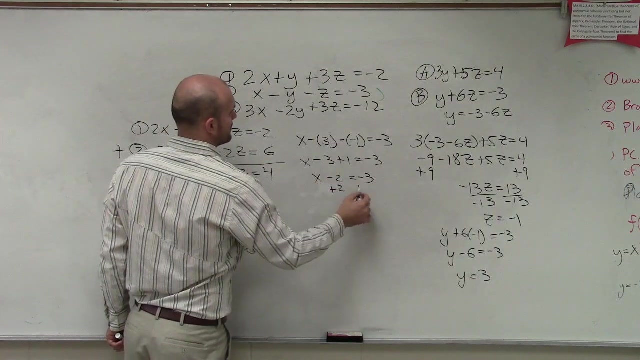 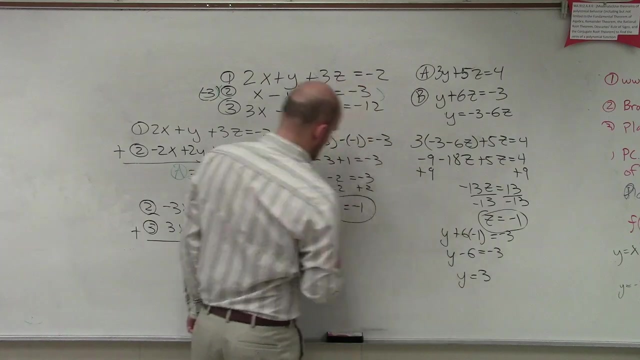 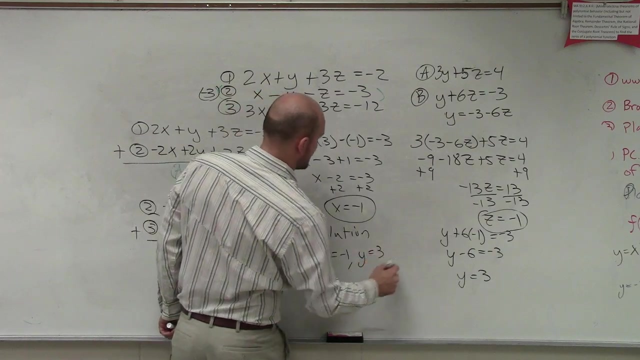 the least amount of exponents. So therefore I have: x minus 3 plus 1 equals negative, 3.. x minus 2 equals negative, 3.. x equals negative 1.. So your solution is: x equals negative 1, y equals 3,. 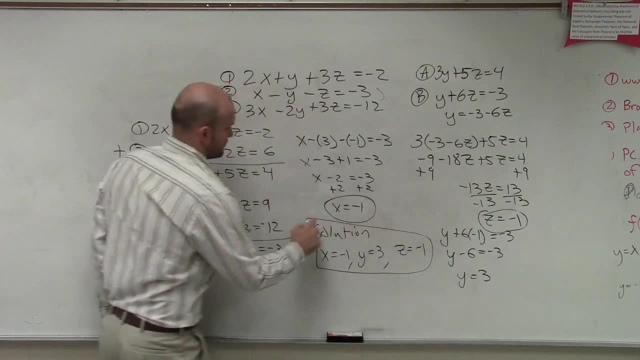 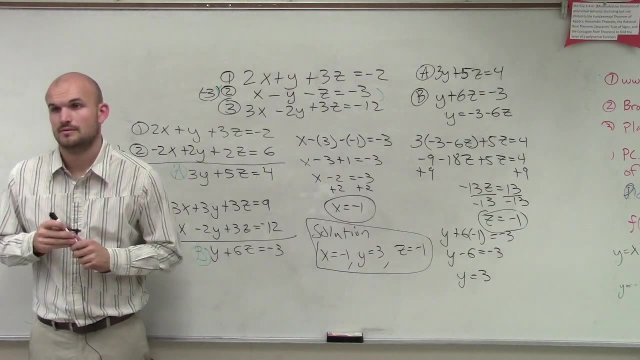 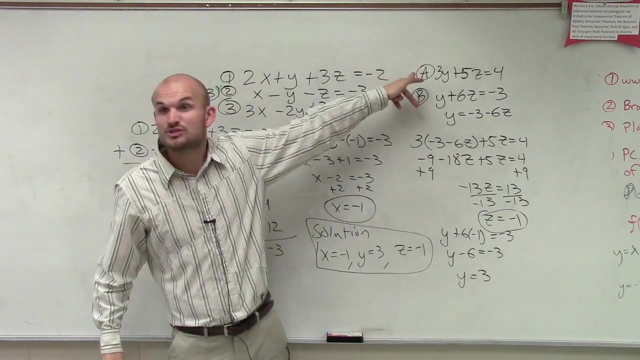 and z equals negative 1.. OK, does everybody see that? See the steps. Yes, When did you guys take a and b and get 1 and a and y? Yeah, we did, We took a and b And what I did was I did substitution. 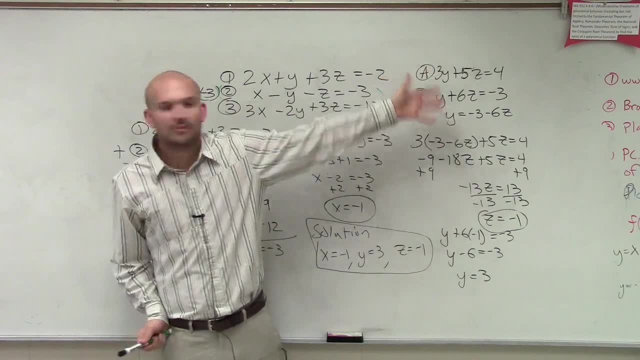 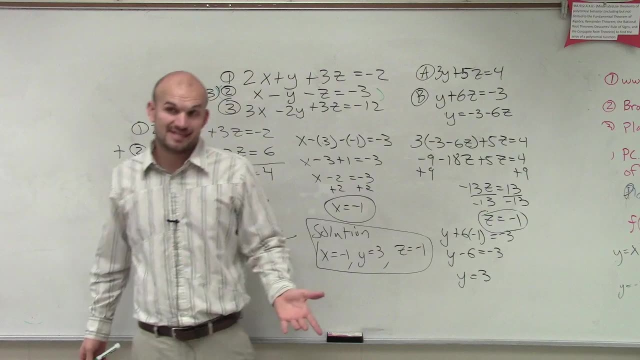 You could have done elimination. You don't have to, though, But I did substitution to get my one variable, And then, once I got my one variable, I plugged it in to find the other one. So if you want to continue with elimination, 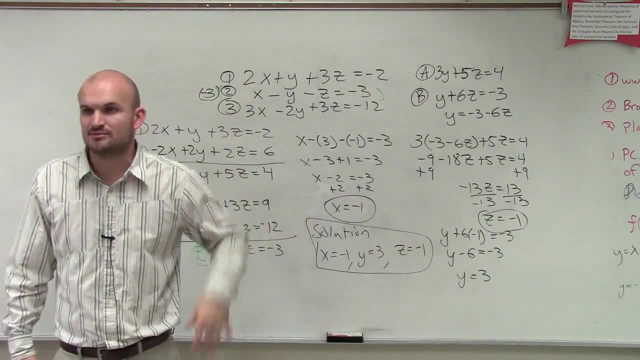 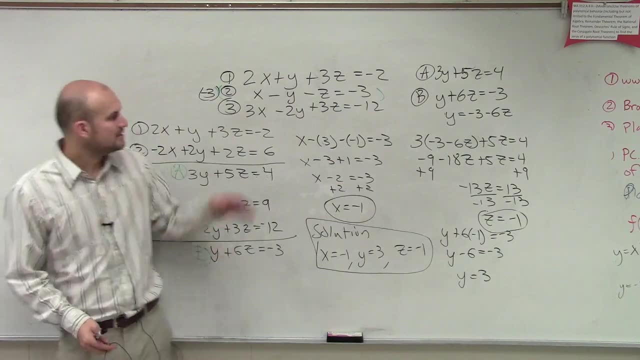 you can do that too. I just decided to get rid of the one variable by using substitution. Does that make sense? What I'm talking about? I just used substitution just to kind of change it up. to remind you guys, you can use both.